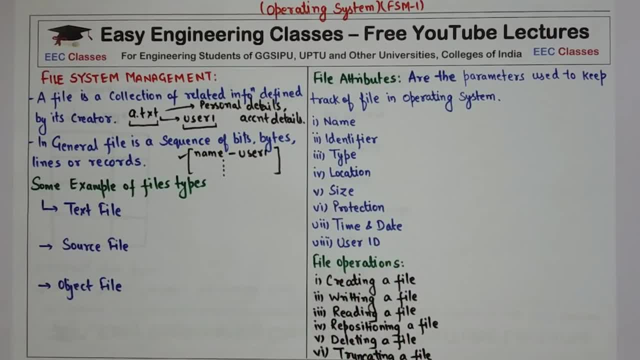 introduction of file. that file is a collection of related information created by its user. Now there are different types of file. some of the example of file types are text file, source file and all the others. So, for example, if we have a source file, we can use this. 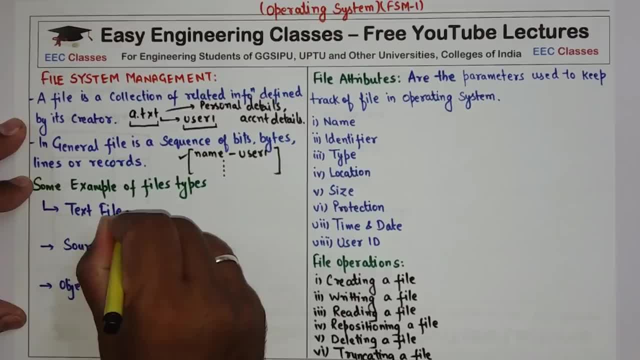 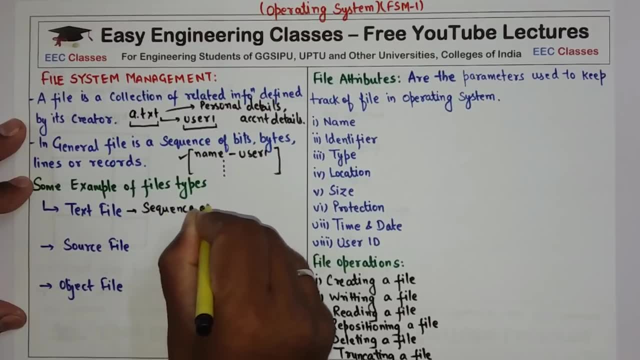 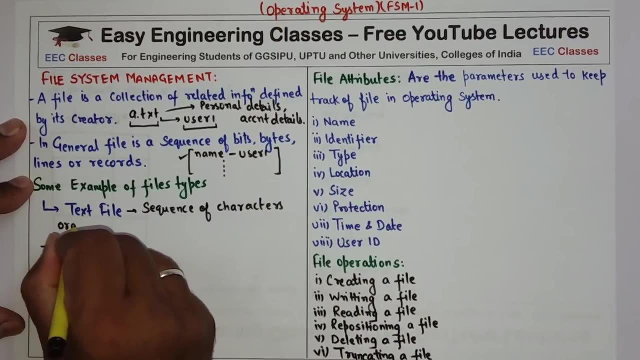 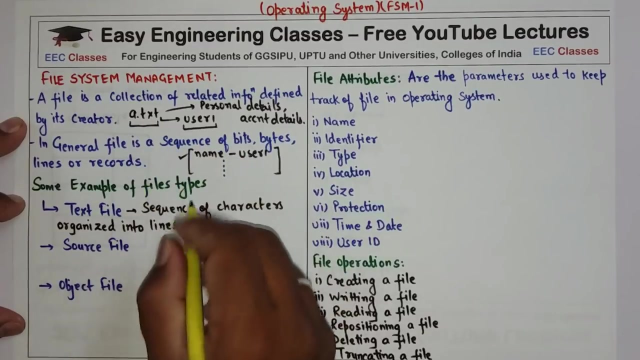 object file. now, what is a text file? as you all know, text file is a sequence of characters organized into lines. you so text file is a sequence of characters organized into lines. for example, this is a text file in which the characters and a, m, e and so on are organized into lines. so this is a simple. 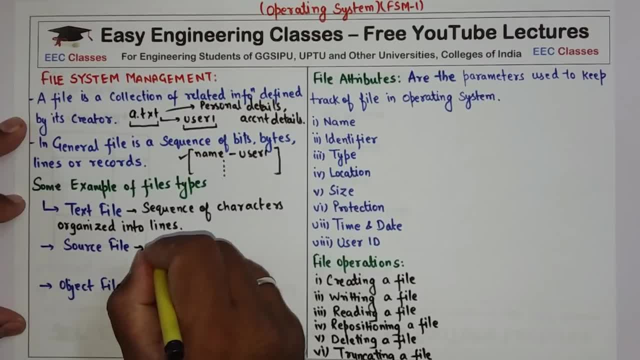 text file, then we have a source file. source file is a sequence of source file is a sequence of subroutines or functions, subroutines of functions which are executable and are defined to work a specific task. So if I say, if I have a source file, say A, and this source file contains two functions, 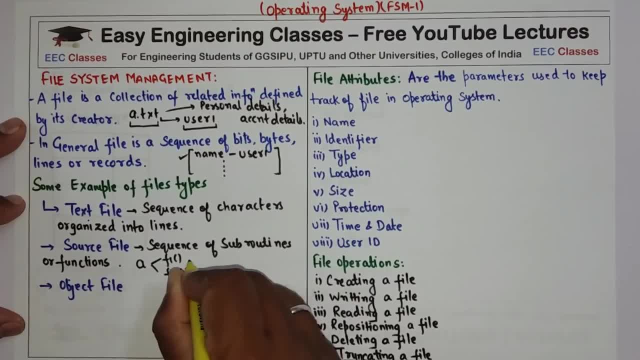 f1 and f2, and f1 is calling function f2 in the source file. Now, if I open this source file, which is an executable file, this function will automatically called and in the middle of this function or in any sequence of this function, f2 function. 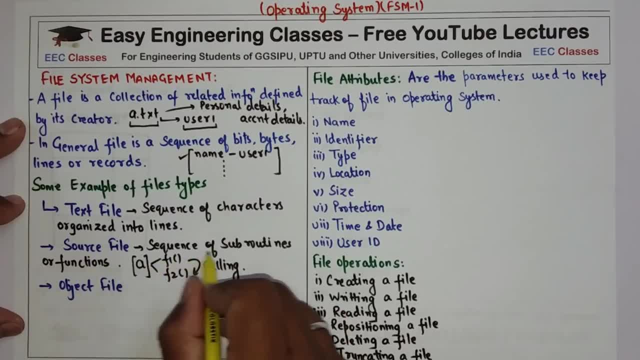 will be called So. source file contains sequence of subroutines or functions which are executable and are designed to do some specific task. Then the next type of file is a object file. This is a collection of words. This is a collection of words. 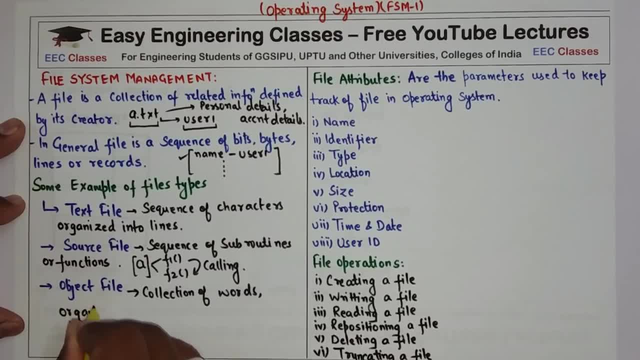 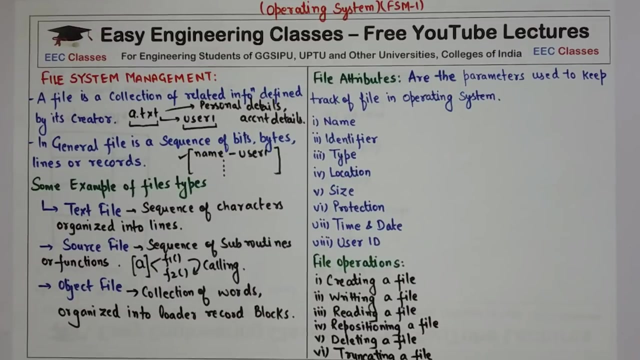 Organized into loads. Organized into loads, So object file is a collection of words which is organized into loader record block. Now, as you all know, that whenever a function, a subroutine or any task has to be performed, there is some loader which gets called and there are certain properties, certain aspects. 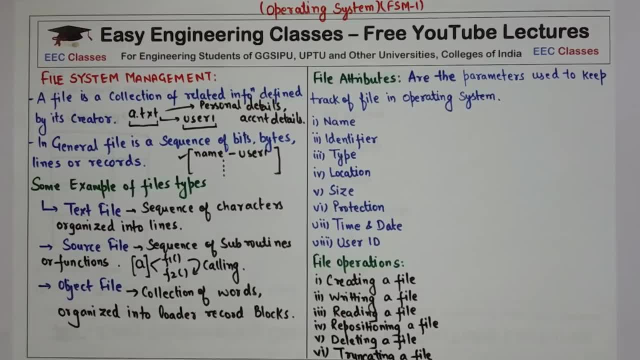 of the function or the subroutine Which needs to be initialized. So generally those properties, those factors we initialize in this object file. So these are some of the example of file types. Now there are different attributes of any file. We are going to study those attributes. 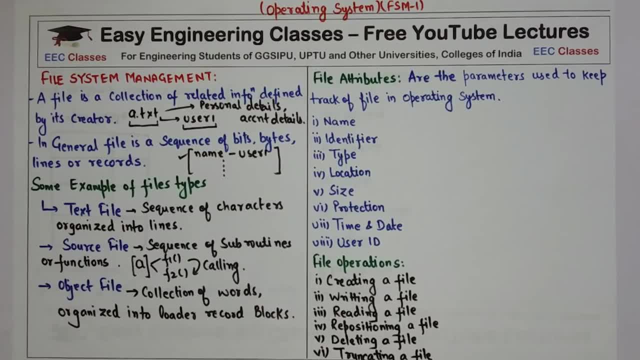 What are attributes first? So attributes are the parameters which are used to keep track of file. So attributes are the parameters which are used to keep track of file. So basically, these are some of the properties of the file. so basically, these are some of the properties of the file which are used to keep the log of the file in the operating. 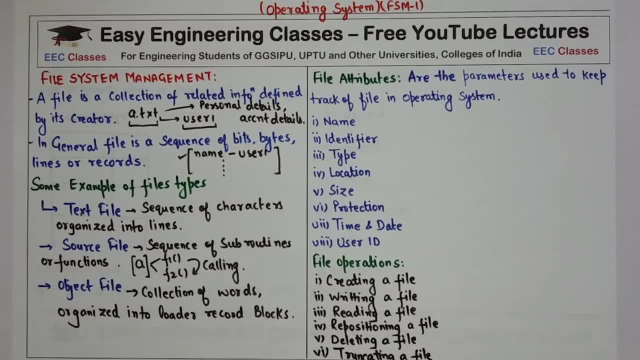 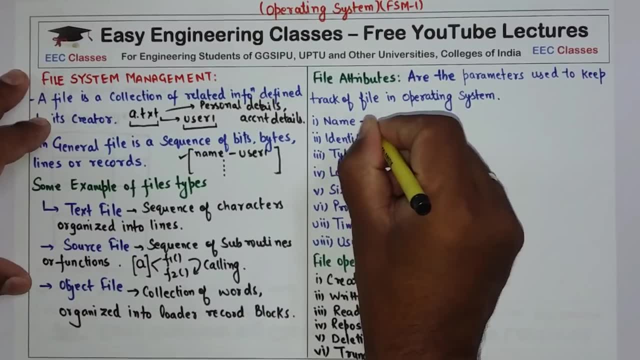 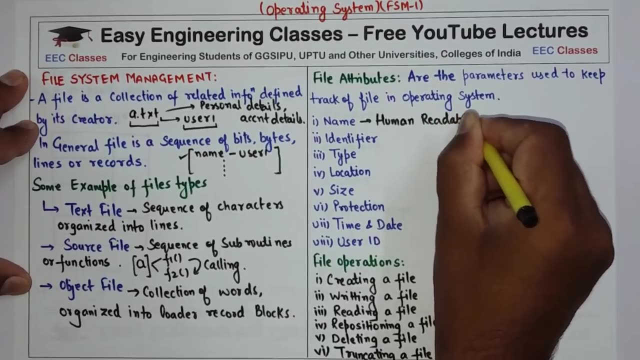 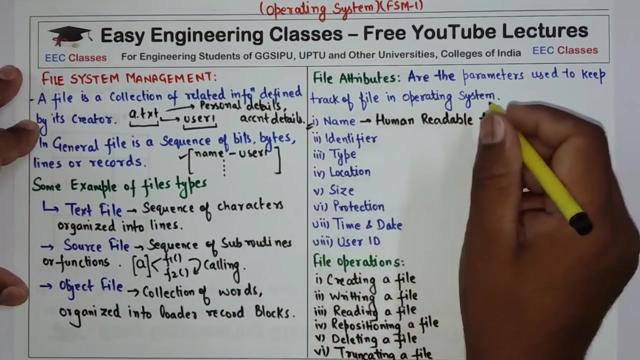 system or record to keep the track of the file in the operating system. So some of the attributes are name, so name is a human readable form, is in human readable form Now. So Name And as per the attribute name, it is clear that it contains the name of the file. 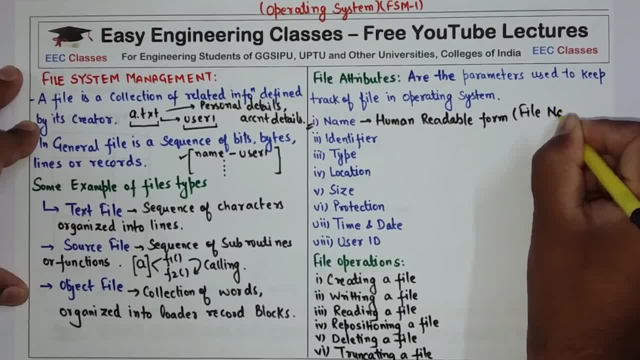 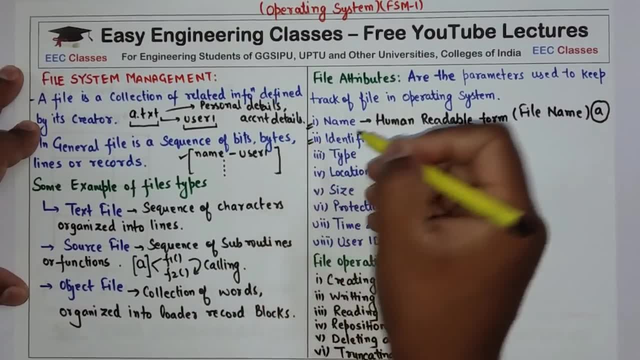 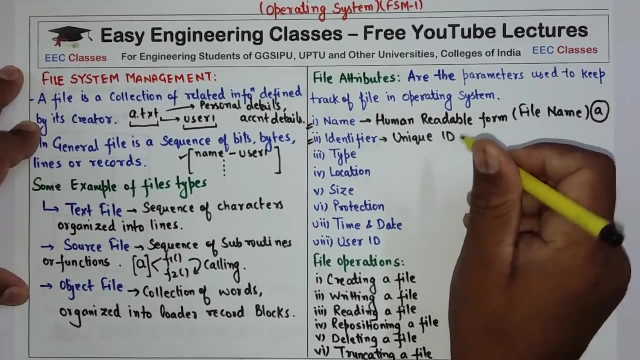 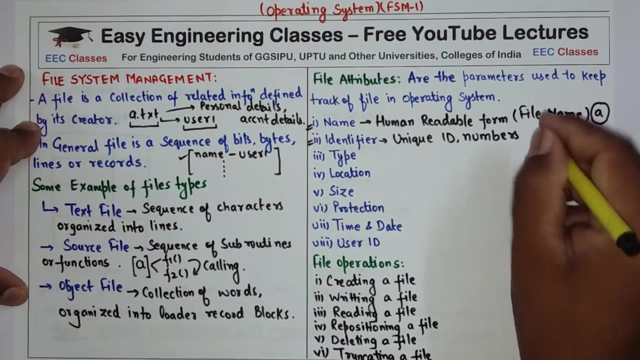 So, basically, it is the file name And, for example, a is the file name. Now, second, we have the identifier. It is a unique id or the unique target, You can say the unique id, generally represented by numbers, generally represented by numbers, and identifies the file within a collection of all the files of the operating system. 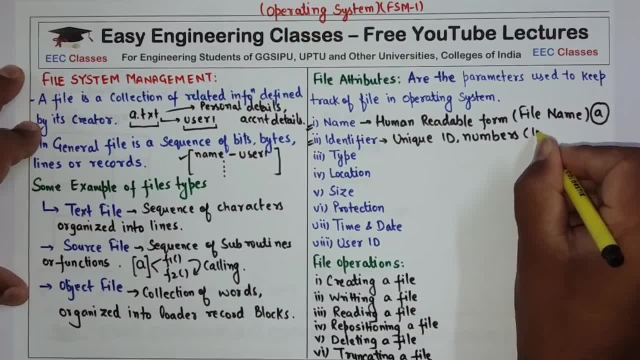 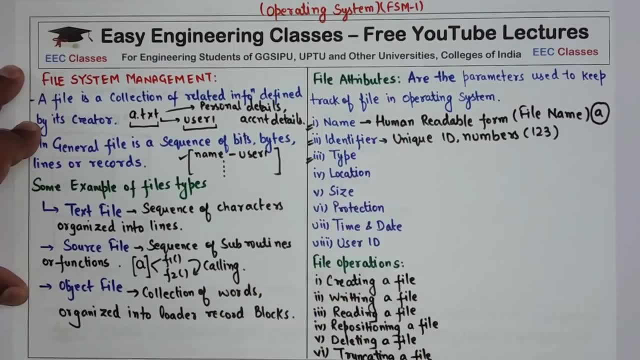 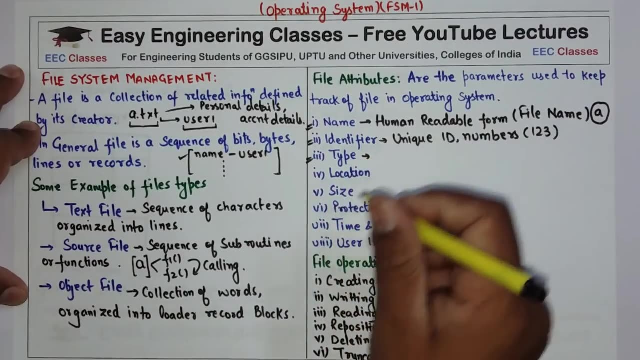 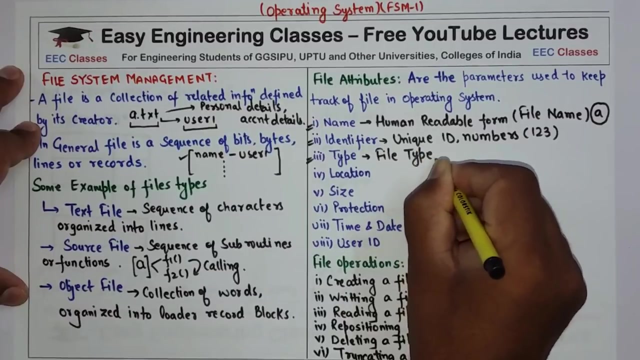 So, for example, if the id for a is 123, so this is the id for the file a. That is your identifier. Now type. It specifies the type of file, So it is the file type basically. So, for example, if the file type of a is txt. 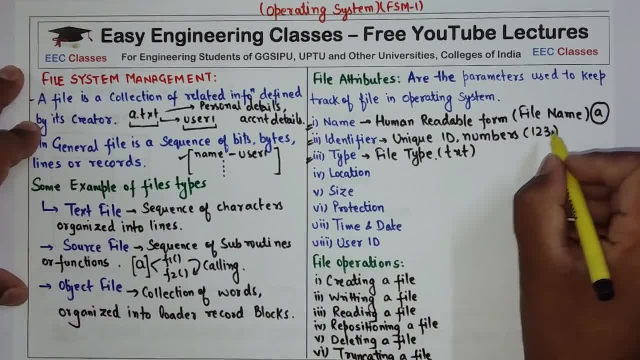 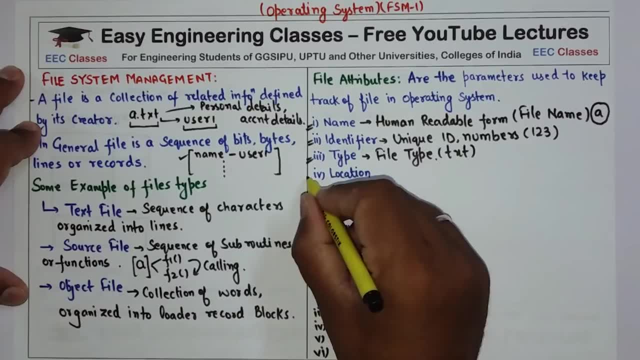 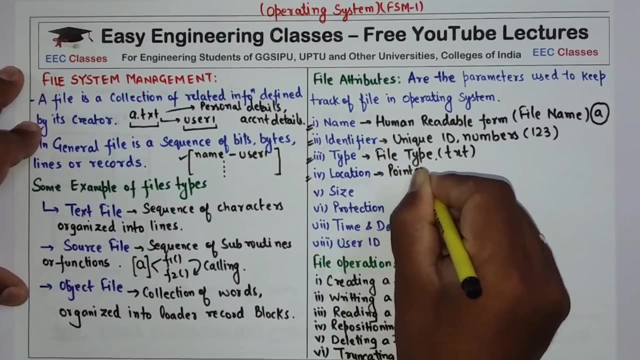 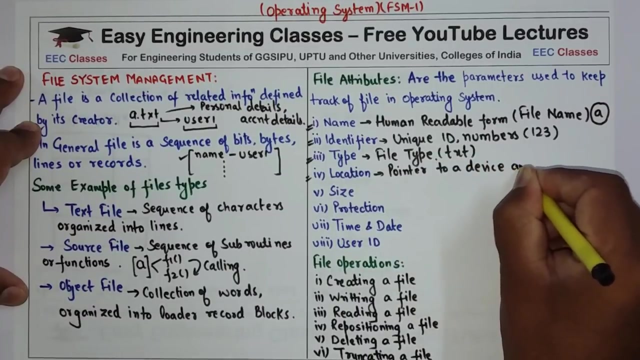 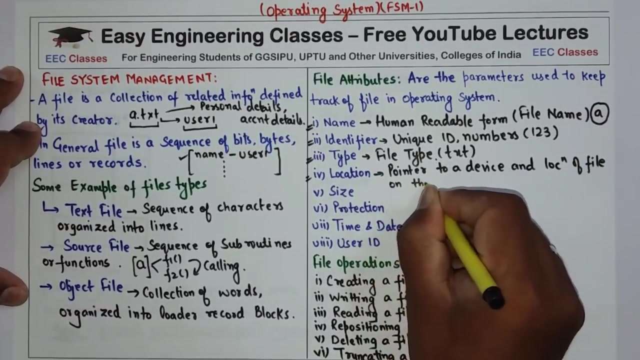 So now I have the information that there is a file in an operating system with the name a, having identifier 123 is of type text. Then the fourth attribute is the location. It is a pointer. It is a pointer to a device and location of file on the device. 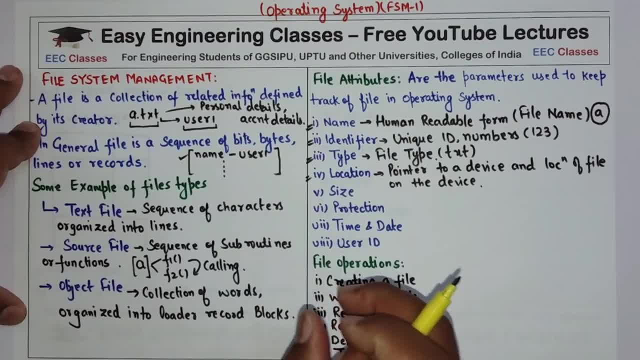 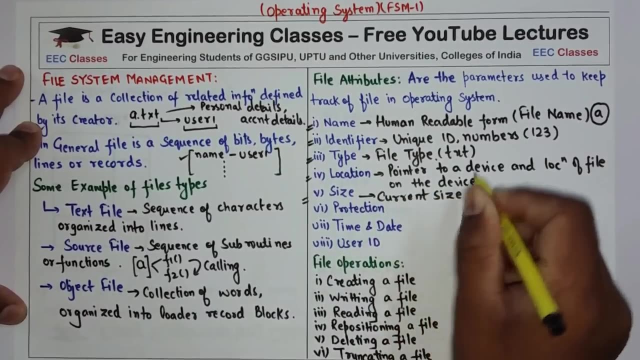 So this parameter, this attribute, is telling the operating system that at which location, at which device the file is stored. Then we have the size. It is the current size of the file. It is the current size of the file. So if I say 1024 kv. 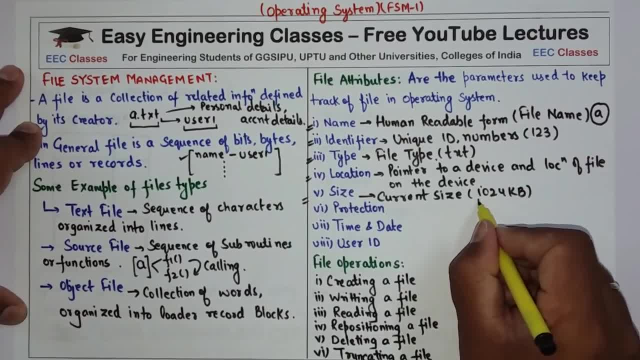 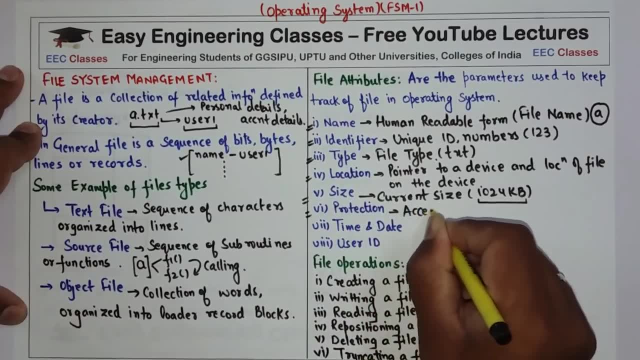 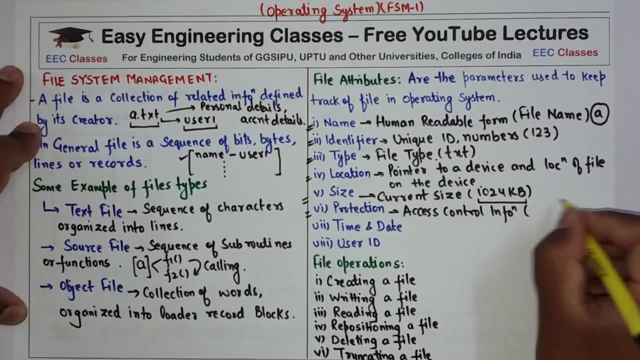 So I have a information about file a having size 1024 kv, Then the protection Protection is the access control information. It is the access control information. Now, If I have a access control information, let's say this is the file name and this is user. 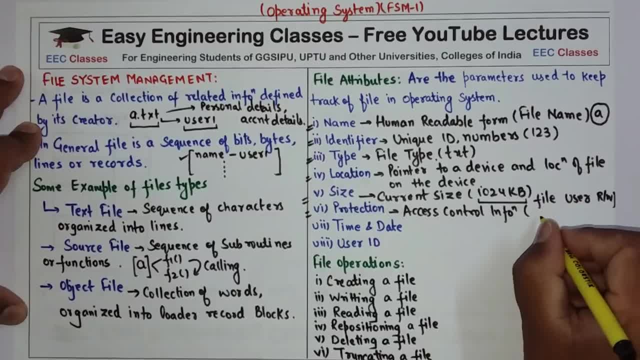 and this is read or write access. So if I have a file user u1 read, So from this parameter I am getting the information that file a can be read by user u1. So it means that user u1 cannot write this file a. 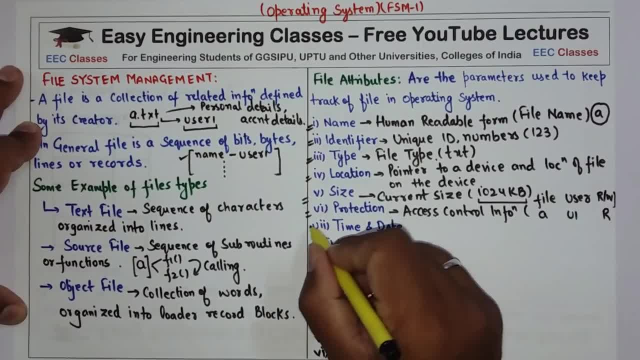 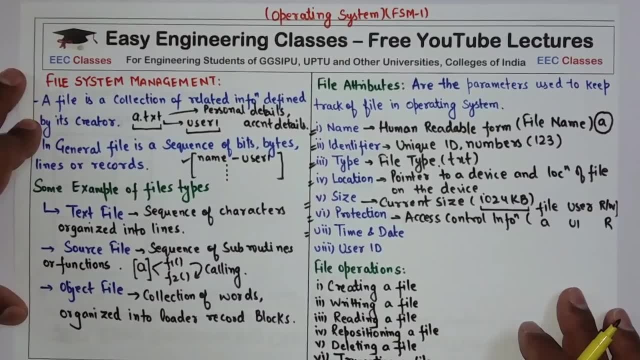 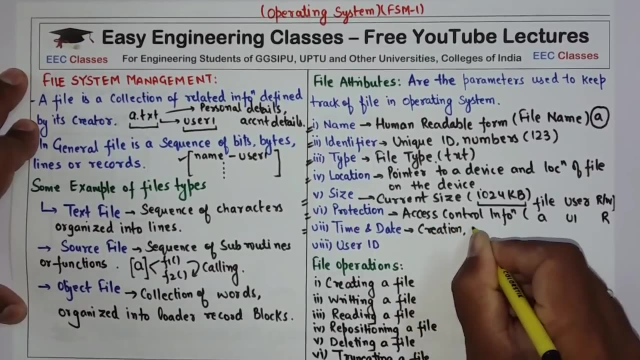 But it can read the file. So like this, you can have different access control information about a file, Then the time and date. This is the information which is used to maintain a log- that when the file is created, So creation, modification, when the file is modified or deletion. 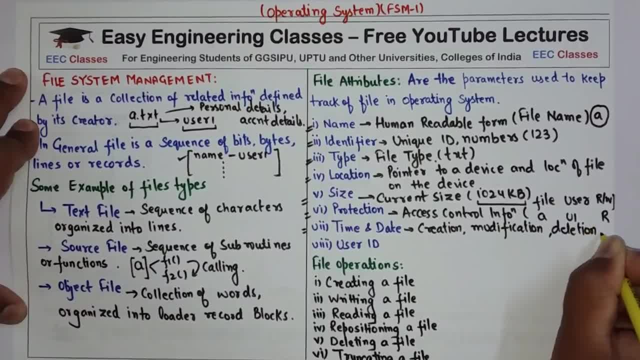 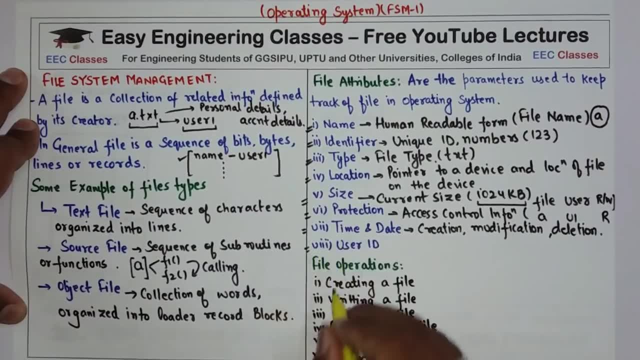 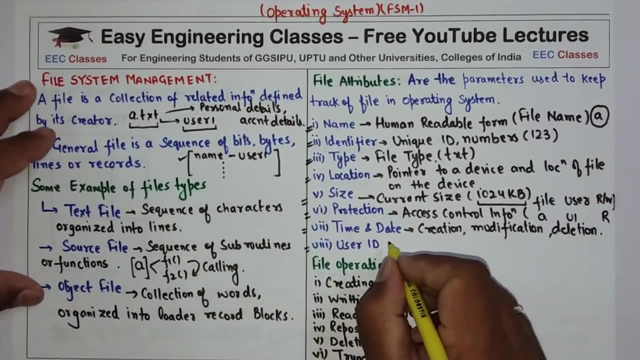 So when the file is deleted, So it gives information about the time and date at which this operations are performed on a file Specified. Then we have the user id. It is the user identification. So user id is nothing but a user identification which is used to give a unique id to the user. 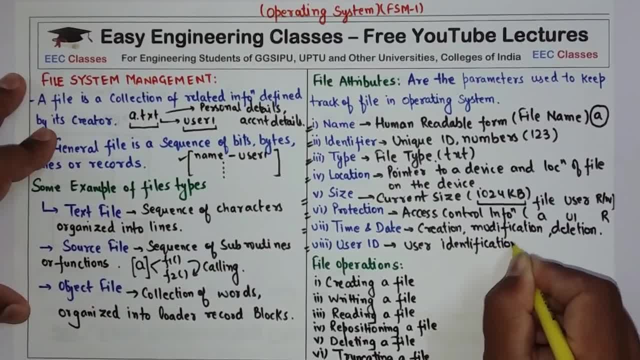 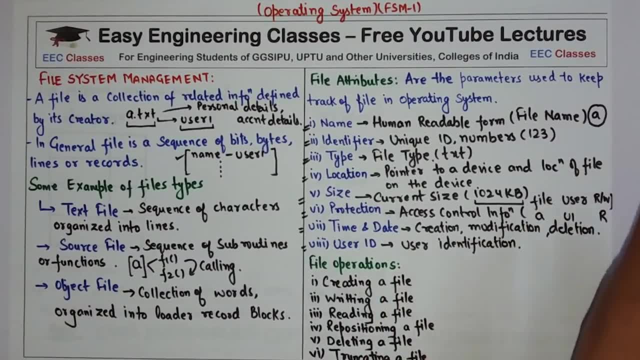 or creator of the file. So these are some of the attributes. So whenever question comes, you can take an example of single file and mention all the attributes in a tabular format. That is all. It will be more presentable and you will get more marks in that way. 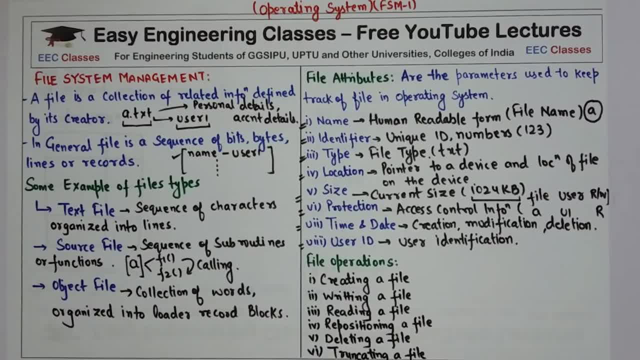 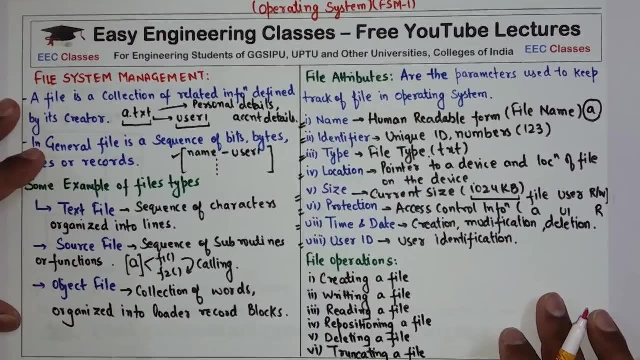 Then there are different operations on the file, So we have file operations. the next topic- It is very simple. First is the creating a file. So to create a file you need to have two steps. One is you have to found the space in the system. 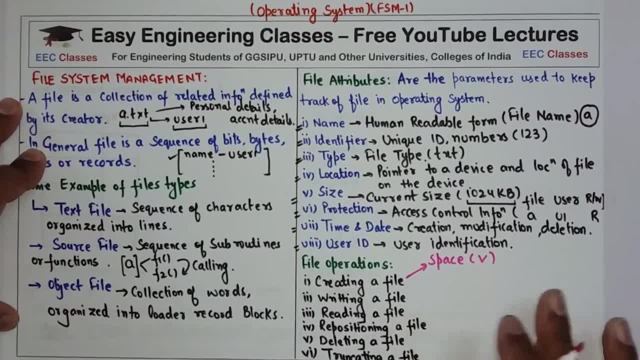 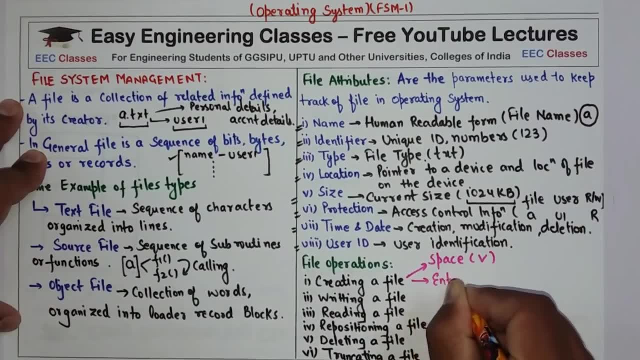 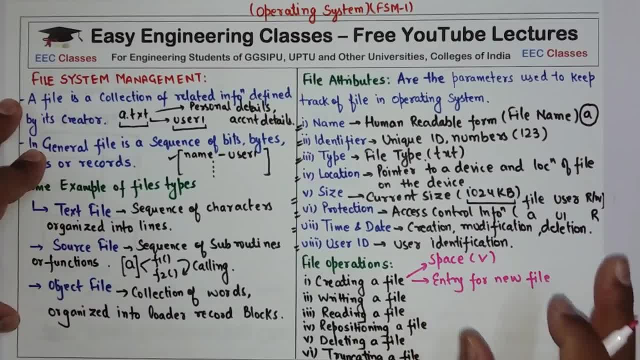 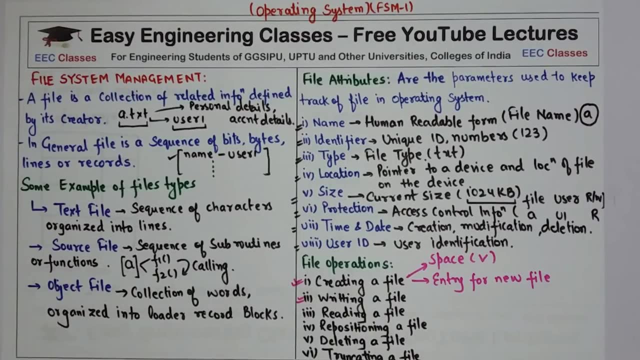 So once the space is found, you have to create a new file and enter that file in the file system. So this is creating a file. Then we have write file. So to write a file you have to make a system call, both by specifying the name of the file. 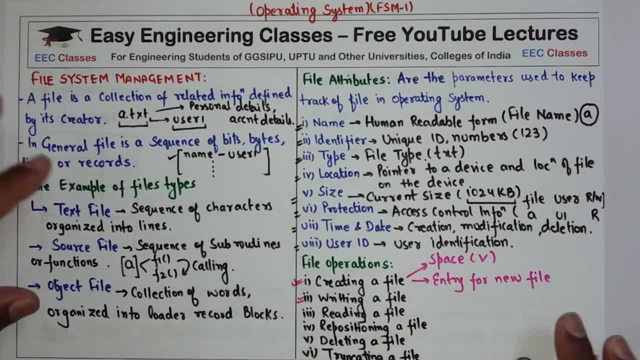 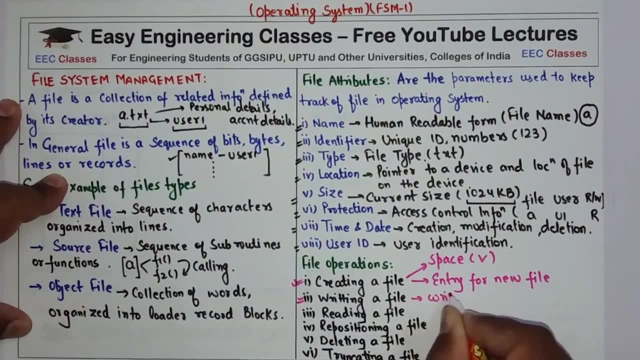 and the information to be written. So if I have to write, for example, in file A, So I can call a system call, for example like this: write A comma AVC. Now this is just an example. this is not exactly the right system call. I am just taking an example that if it is a system call, write it is telling me that. 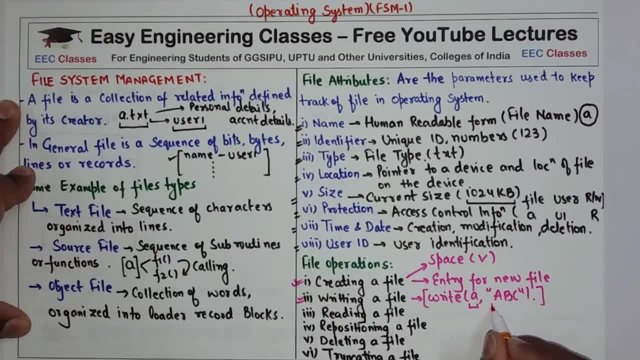 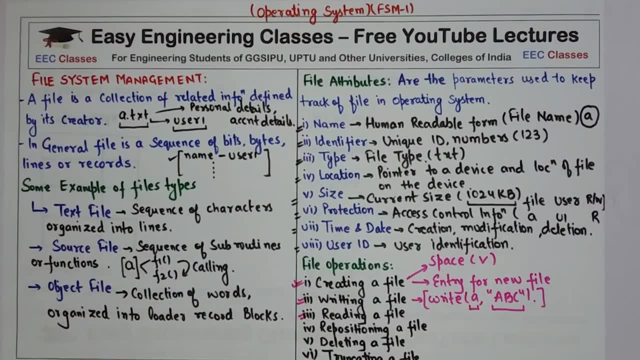 I have to write to file A and the content that needs to be written is AVC. That is your writing a file, Then reading a file. Now to read a file, a system call specifying the file name and when the next block of the file should be put in the memory.